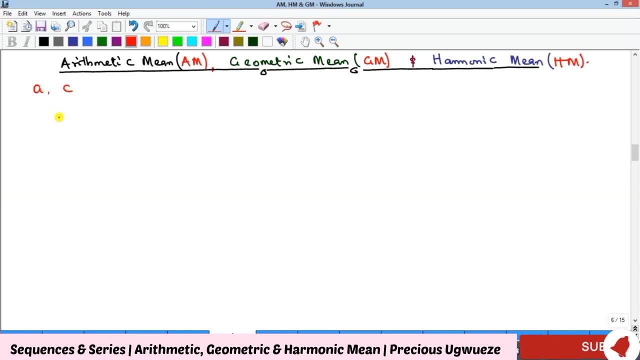 say A and B- sorry, C- as two elements in a sequence. Now the mean of these two elements is another element that will come in between them, let's call it B. That will come in between the two of them and it will still give you three consecutive elements of, say, arithmetic. 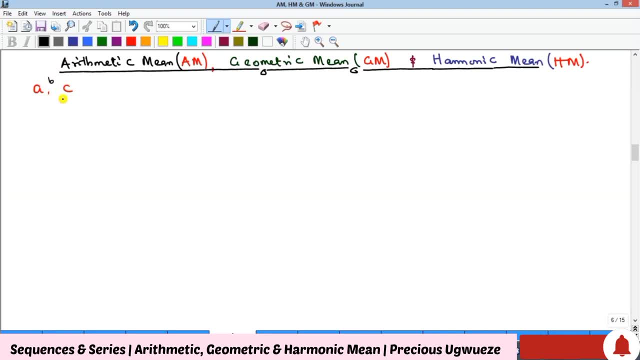 progression. So if it gives you, let's say, A, C are in terms of an arithmetic progression, and then you introduce b and you still have three consecutive elements of an arithmetic progression, then you say that b is an arithmetic mean of a and c. and if it happens in a geometric progression, 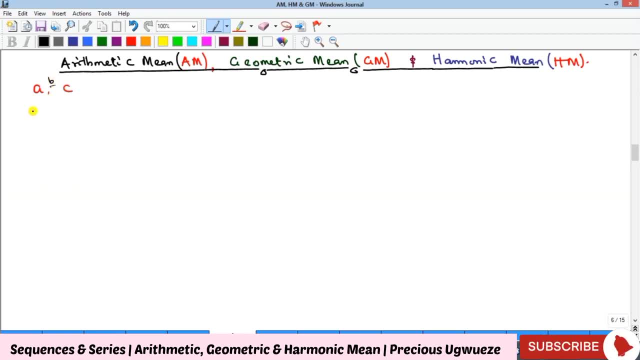 you call b the geometric mean of a and c. that means you introduced it in between a and c and you still have three consecutive terms of a, gp. and then, if it happens in harmonic progression, you call it harmonic mean. all right, now if it is for arithmetic mean, now how do you get that b? we? 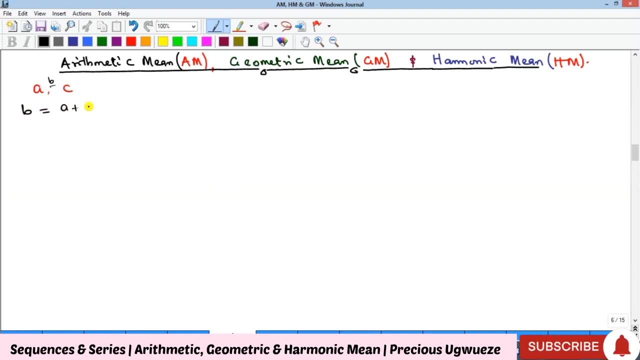 said that that b is equal to a plus c, all over two, and we're going to see how this is gotten. and then, what about geometric mean? now, your geometric mean. b is always equal to the square root of ac. and then what about the harmonic mean? so your harmonic. 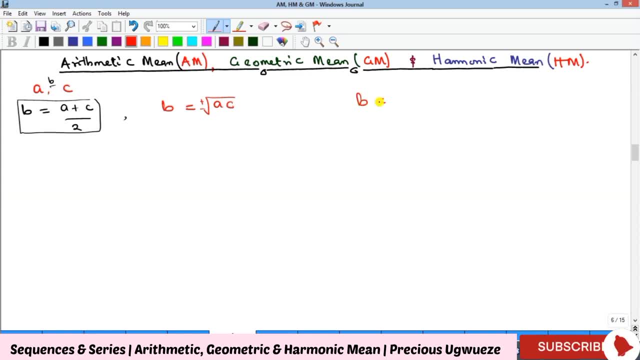 mean b is always equal to the square root of ac. and then what about the harmonic mean? so your harmonic mean b is always equal to the square root of ac. and then, what about the harmonic mean? so your mean b is that element- that is you- that you can get when you have 2ac all over a plus c. 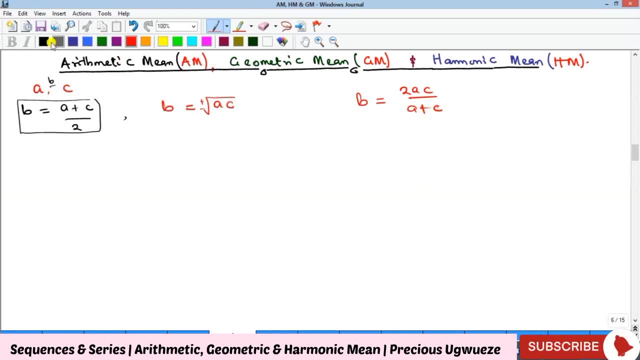 all right. how did we get all of this? now you recall that let's say you have two terms, a and c, and then you decide to introduce b, and there is one thing that defines an arithmetic progression. that thing is that you must have a common difference. so what it means is that b minus a 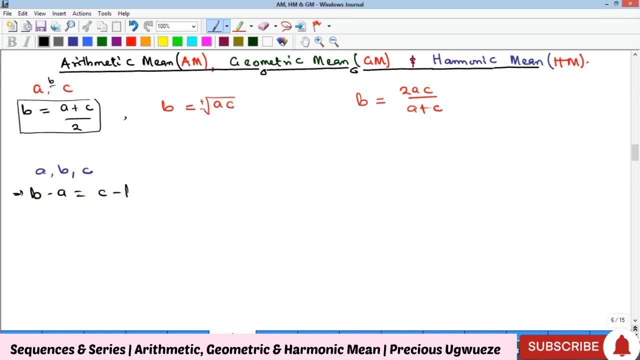 must be equal to c minus b. okay, so from this equation we can find our b. you are going to have b plus b, which is 2b, and then a coming here will give you a plus c, and so therefore, that's, we got b to be a plus c, all over 2. all right, which is the the arithmetic mean. and then what? 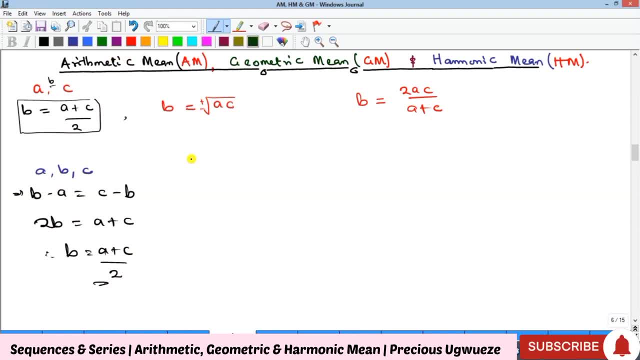 about the second one for geometric mean. so you recall that when you have a, b, c, adiabatic, And we said that the three of them are three consecutive terms of a GP, And so you also have the concept of your common ratio. So the implication by common ratio is that B, all over A must give you common ratio. 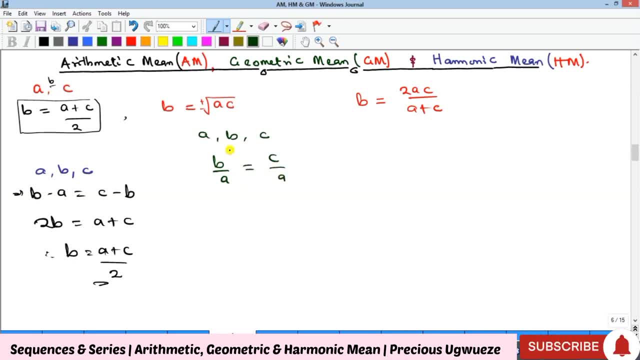 which must be equal to C all over A. That means, sorry, C all over B. Alright, so, and then when you make B the subject of the formula here, what will happen? You are going to have B squared. that's cross. multiplying B squared is equal to AC. 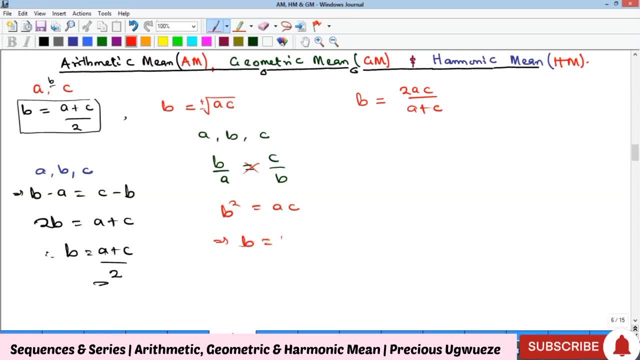 So, which means that B alone is equal to the square root of AC. Now, one condition that you must note here is that for a geometric mean to be defined, the symbol sign for the two terms you want to define a geometric mean on- must be the same. 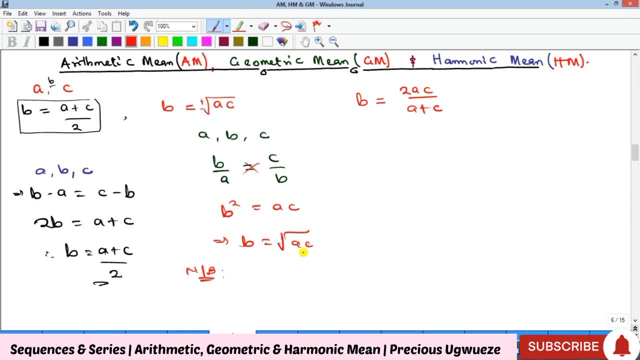 They must be either both positive or both negative. That's your A and C. Please take note of that. And then, how did we get the arithmetic, the harmonic mean? Now you recall that if A, B, C are in consecutive terms of a harmonic progression, 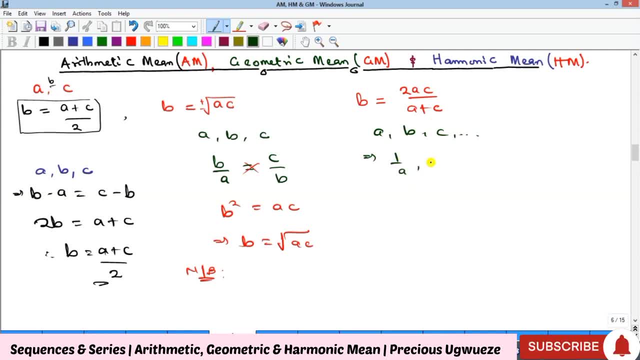 what it means is that 1 all over A will be in arithmetic progression. You recall the reciprocal will give you AP, And so by this same condition here you are going to have that 1 over B minus 1 over A must be equal to 1 all over C minus 1 all over B. 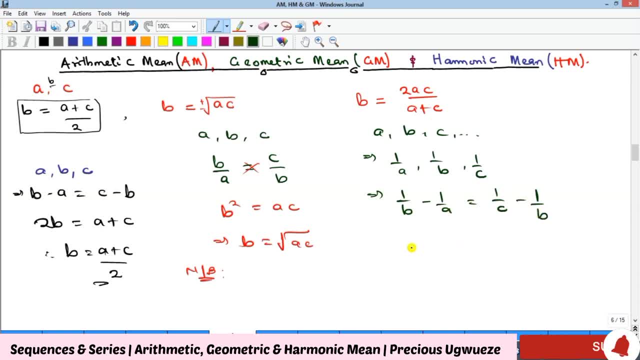 And so if I take this to this side and this one, this one, I'm going to have 2 all over B. That's this plus this, And then that is going to be equal to. So if we decide to now take LCM here, we are going to have AC and this is going to be, of course, A plus C up here. 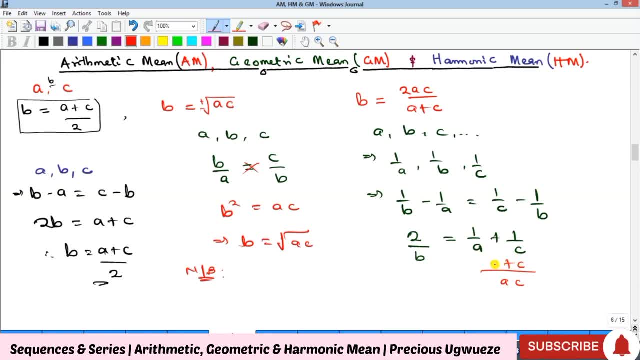 That's if you rearrange it. Of course you're going to get C here and then A here, But if you rearrange it we'll have this Recall that this is 2 over B, And so from here, if we cross, multiply and then make A the subject, we are going to have, sorry, B. 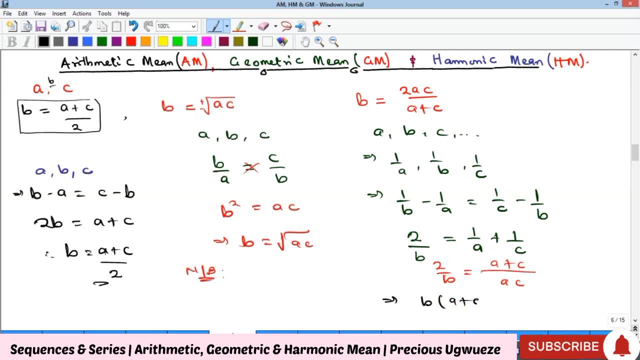 We're going to have B. multiplying A plus C is equal to 2AC. All right, And so if you divide both sides by AC now, you are going to get this All right. So that's how all of these formulas were gotten. 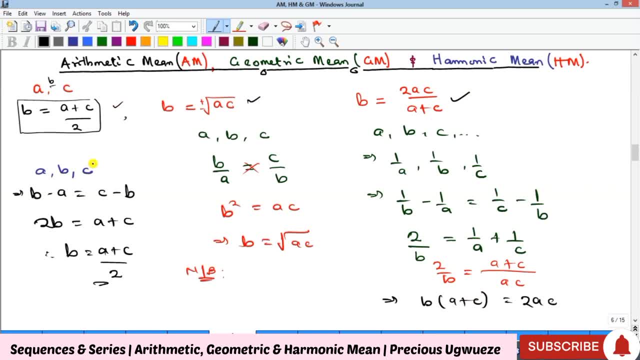 And please note that you can actually make use of the mean to check the nature of a sequence. So In case you are asked to determine whether a sequence is an arithmetic sequence, you can just use the mean, Just pick any two, any three consecutive terms in that sequence. 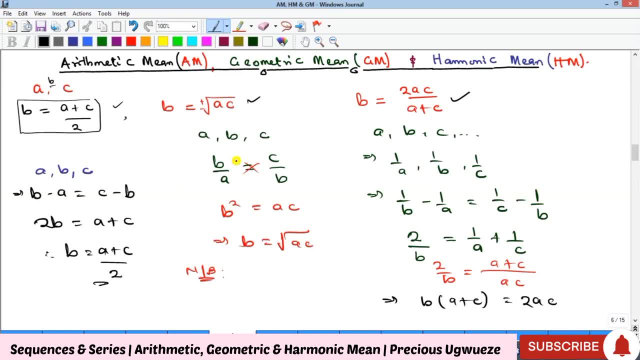 And then use the last, the first and the last, to form your A and C And then use this formula to check if you get the middle one, And then you can do it for this and do it for this. For instance, in our previous video I said that if you have 6,, 4,, 3.. 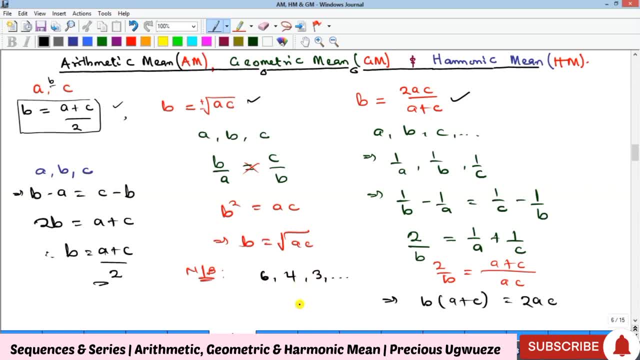 That this, This is a harmonic progression, So we can check with this formula if that is true. So let's see. The implication is that this is our A and this is our C, And so what it means is that if we have 2 times our A, which is 6, times our C, which is 3.. 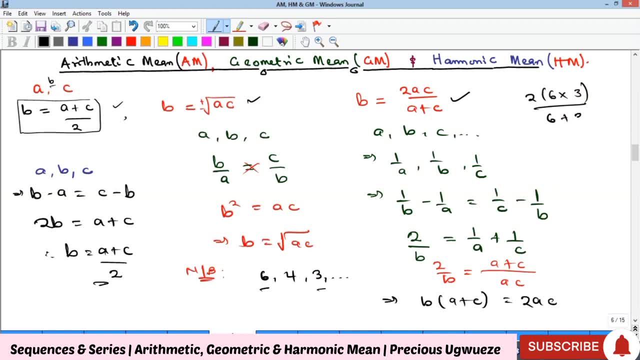 And that is all over 6 plus 3. That we should be able to get the middle one, which is our B, And of course you can see this is 18.. And 18 times 2. Is 36.. All over. 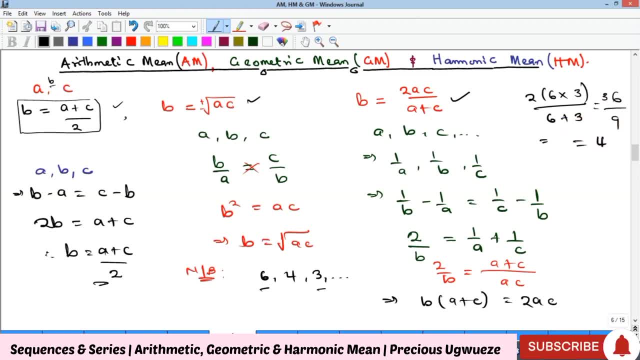 This one is 9.. 36 over 9 is definitely equal to 4.. Alright, And that proves that this is actually a harmonic sequence. Okay, So now we are going to take some examples. How does this concept here help us in solving problems? 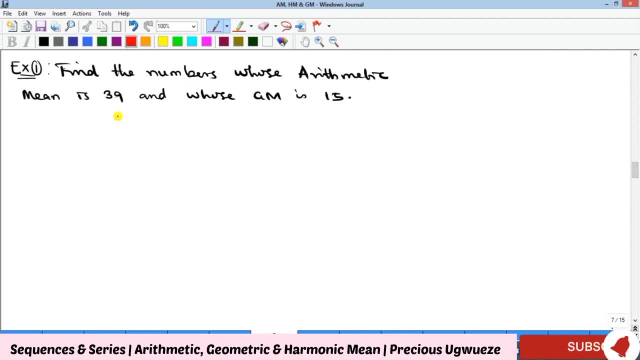 Example 1 here says that we should find the numbers whose arithmetic mean is 39.. And whose geometric mean Is 15.. Okay, So what it means is that you have 2 numbers, Let's say AC, And then they are saying that the arithmetic mean of these 2 numbers is 39.. 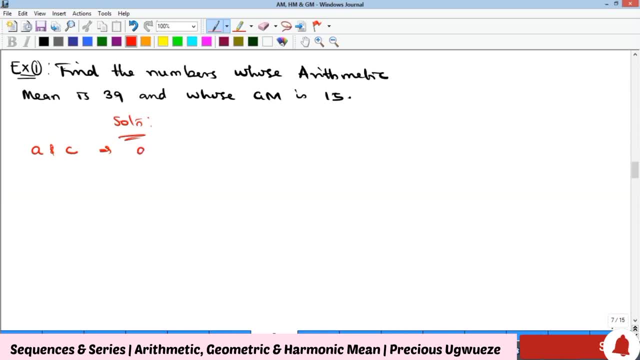 And so what does it mean for the arithmetic mean to be 39?? It means that A plus C, all over 2, must be equal to 39. And so if we decide to push this further, That's going to give us that A plus C. 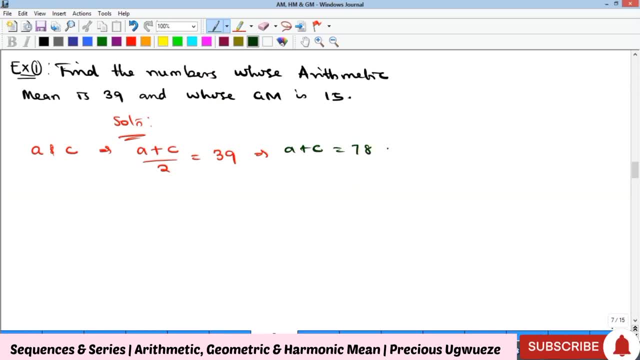 Must be equal to 78.. You can call this equation 1.. And then what's the second information? The geometric mean of these 2 is 15.. So that means that A times C, If you take the square root of it. 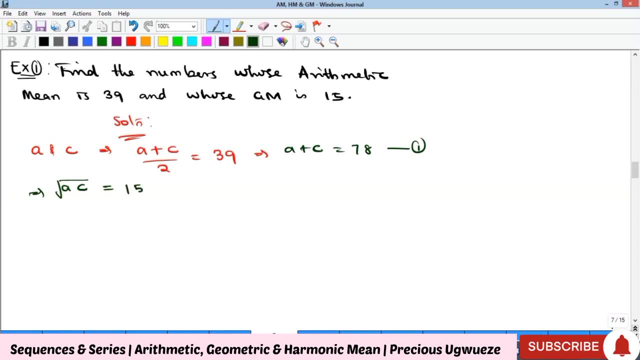 You are going to get what? 15.. Alright, And so what this means is that if you take this square root to this side, You are going to get that AC Must be equal to square root. coming here becomes square And the. 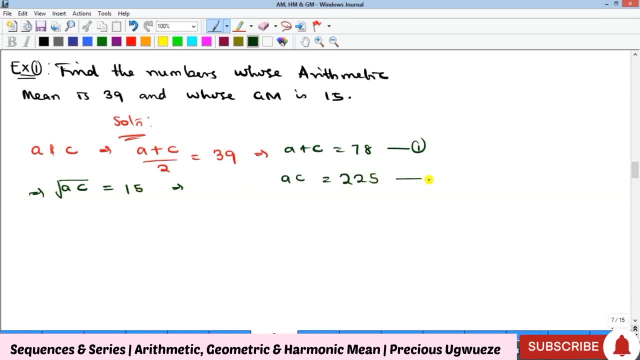 Square root of 15 is 2 to 5.. And so you are having these 2 equations. And they said that we should find the 2 numbers, Meaning we should find A and C. Alright, So we are going to solve that simultaneously. 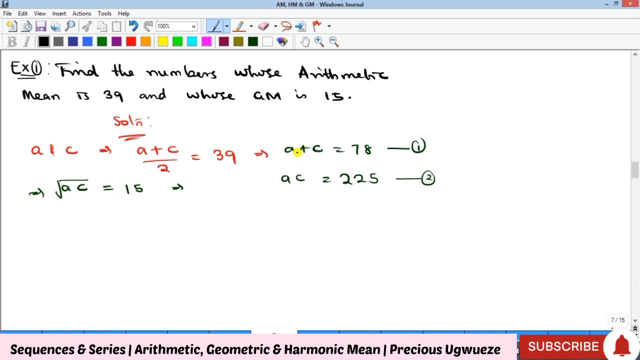 And to do that you can either make A the subject here or anyone. So let's make C subject in equation 2.. From equation 2, you will see that C is equal to 2 to 5 over A, And so if we substitute it into equation 1.. 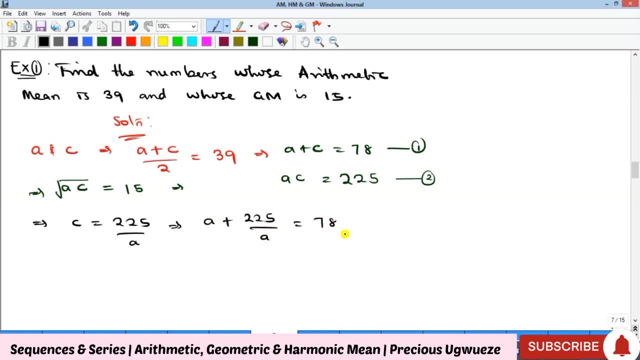 We are going to get. We are going to have A. Okay. So if we decide to multiply through by A, We are going to have that A squared Plus. if you multiply here by A, You will get 2 to 5.. 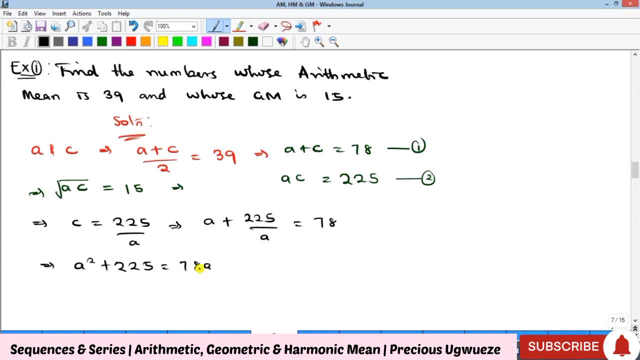 And that is equal to 78A. Okay, So if we take this to this other side, We are going to form a quadratic equation Which is going to give us Alright. So, solving this quadratically, We are going to have: 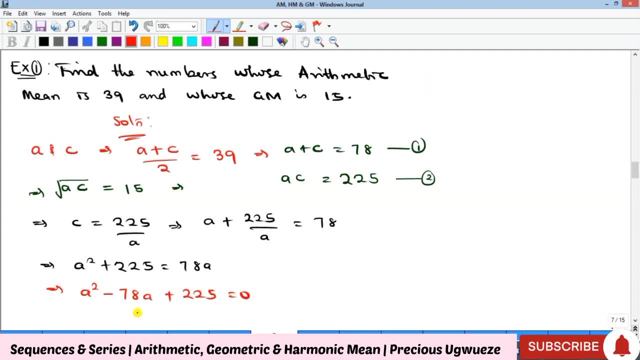 Of course, by factorization method, The two factors here are going to be minus 75 and minus 3.. Alright, So if we bring that here And that is equal to 0.. So, which means that our A is either equal to 3 or what? 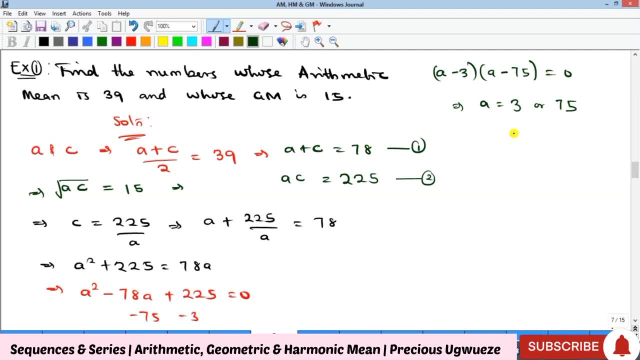 75.. Okay, So, and that is the value for our A, And then to get the value for our C, Just put it into any of this equation. So when A is equal to 3.. If you put it here, 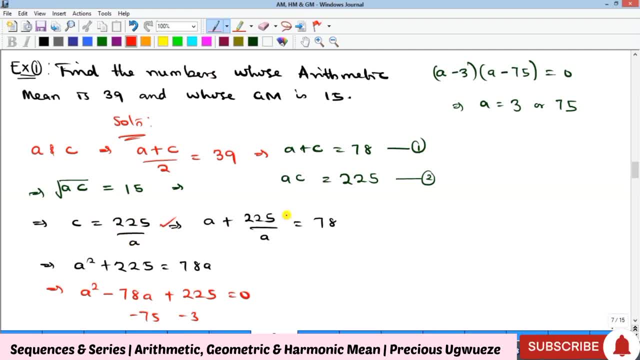 Look at our C here. Sorry, If you put it here now, Then your C 2 to 5 divided by 3 is going to still give you 75. And when A is 75. Your C will be 3.. 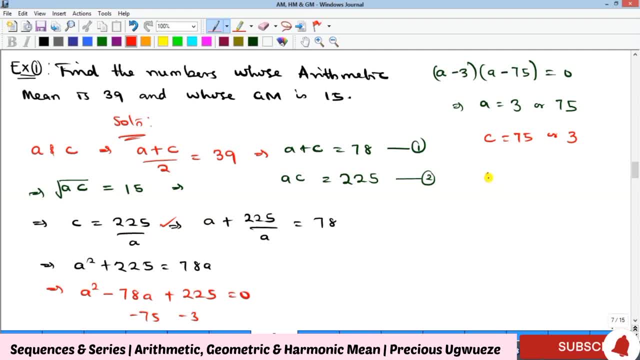 So the two numbers are basically 3 and 75.. Alright And so, and that is our solution to this problem, Of course, if you check it, You see that it is true If you have 3 and 75.. 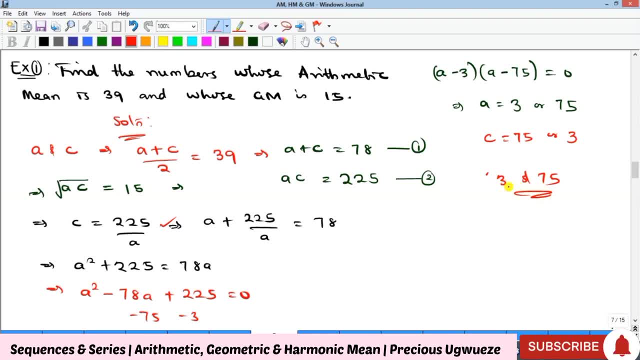 The mean Arithmetic mean of these two: Add the two, You get 78.. Divide by 2. You get 39.. The geometric mean: Multiply the two, You get 2 to 5.. Take the square root And you get 15.. 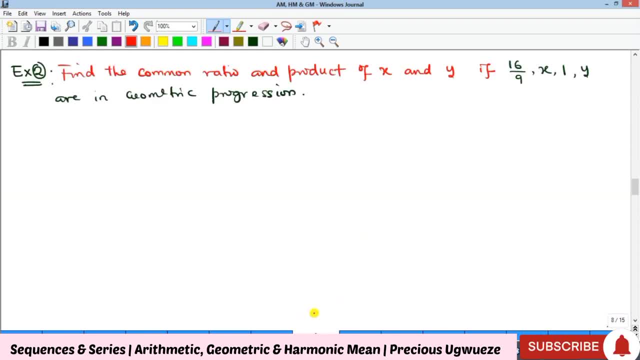 Alright, And that is the solution for that. So what about the second problem here? In this case, We are asked to find the common ratio of this sequence And then the product of X and Y, And you can see, We are going to apply the knowledge of arithmetic mean. 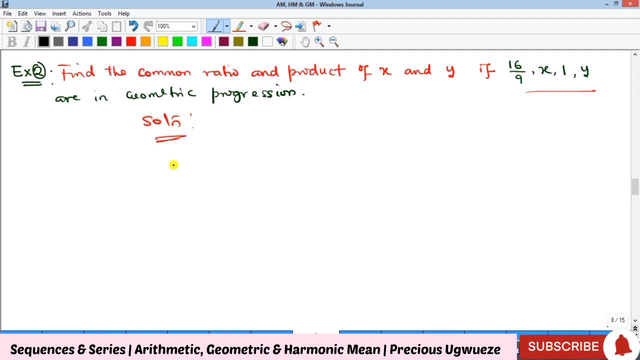 And sorry, In this case It is geometric mean We are going to apply. And what is that? Remember, We are looking for the common ratio. And to find the common ratio, We need at least to find the value of X. 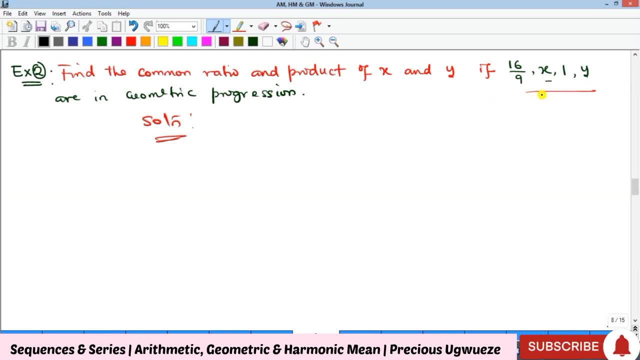 Or the value of Y. If you know the value of X, Divide it by this. That will give you the geometric, Yeah, The common ratio. Sorry, And so. And to get the value of X, We know that. these three now. 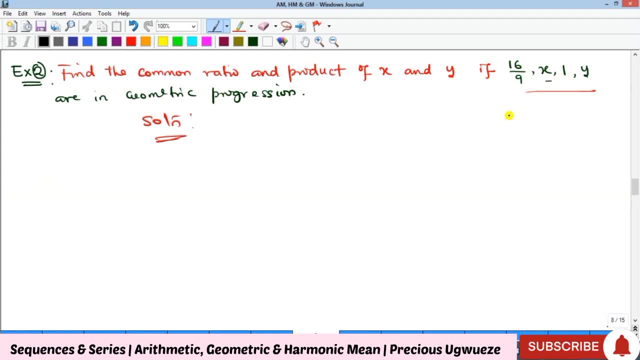 Are three consecutive terms And since there are three consecutive terms, So let's treat this as our A, And this as our C, And this one as our B, And we recall that B is equal to The square root of AC. 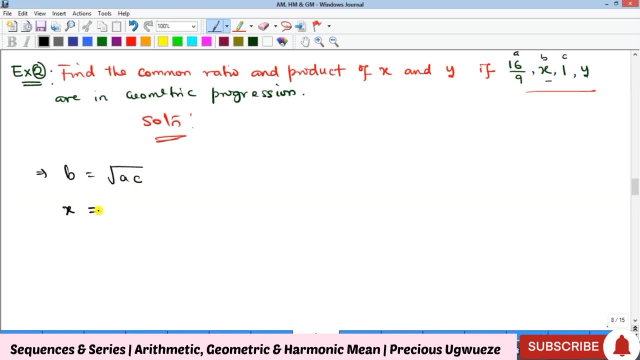 And so in that case, Our B represents X, Which is equal to the square root of A, Is 16 over 9.. Multiply by C, Which is 1.. So you still get 16 over 9.. Therefore, our X alone. 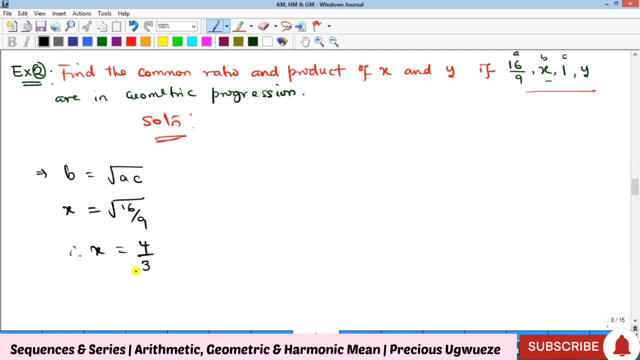 Is 4 all over 3. If you take the square root of this, And so what that means Is That our B is this, Sorry- Our X is this, And so the implication Is that our common ratio, Which is actually. 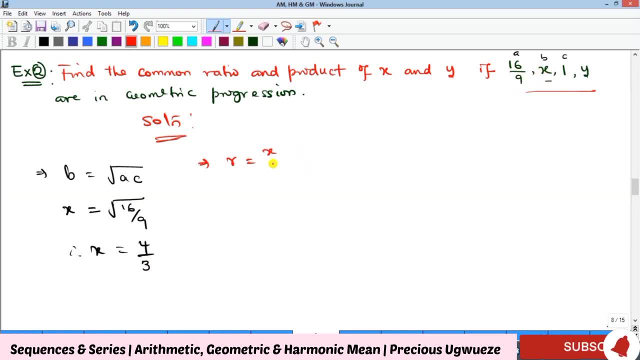 X does. a term Divided by the previous term Is going to be X all over 16 over 9. And if you do this, Our X is 4 over 3. Divided by 16 over 9. If we change it to multiplication, 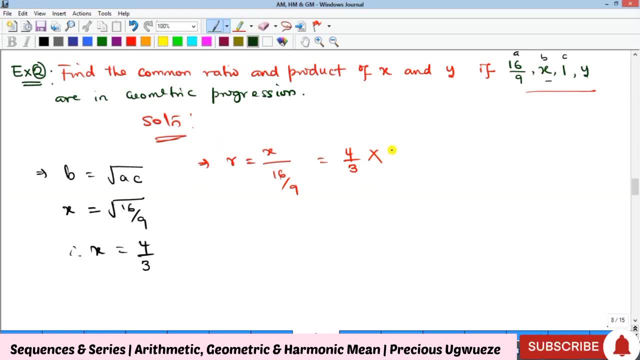 They will invert. So you are going to have, Divided by Sorry, Multiplication, Multiplication Divided by 9 over 16.. And this is going to give us 3 here And here we are going to have 4.. 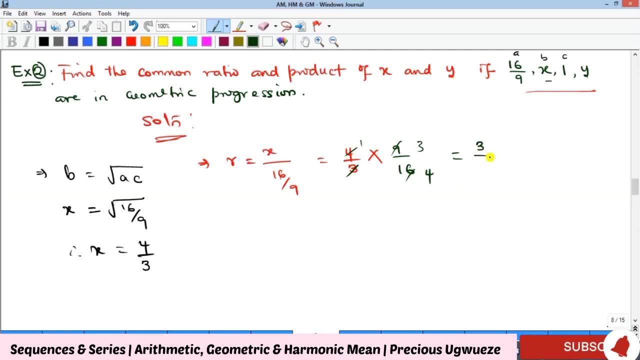 So that means Our common ratio Is 3 all over 4.. And of course, If you say 1 divided by 4 over 3. You still get this Alright. So that's the value for the A part Which is a common ratio. 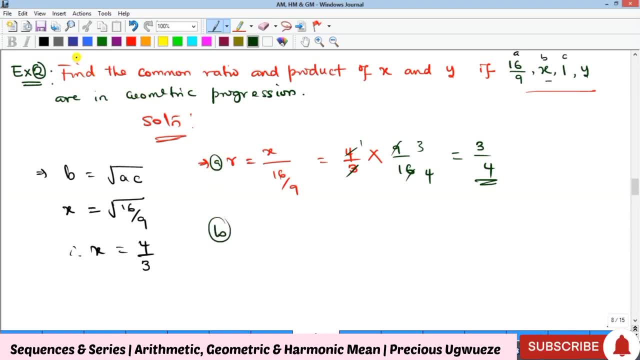 And then the B part. We are asked to find the product Of X and Y, And you will also apply, You know, The knowledge of geometric mean. So in that case We want to call Our X here A And our Y. 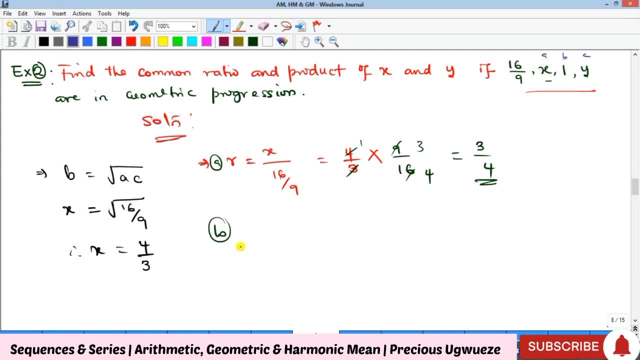 C. So where B, here Is our 1.. Okay, So we recall that By that formula, B squared Is equal to the square root Of A- C, And so that means 1 squared Will be equal to the square root. 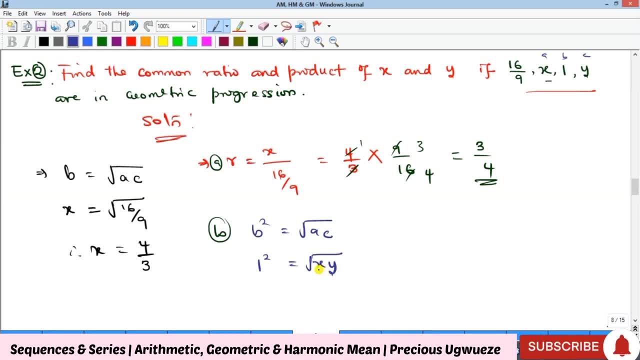 Of A is X, Multiplied by C, Which is Y. So And that is going to give us That 1 squared. If this 1 goes over here, It becomes square root. Square root of 1 is 1.. 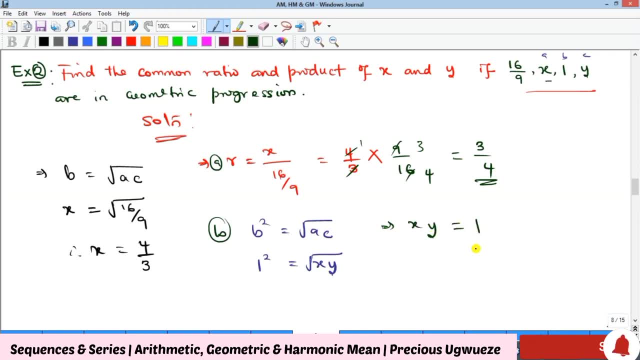 Therefore, A X times Y Is actually equal to 1.. Very simple, And that is The solution For the second Problem. Alright, Let's look at the next example. Okay, So here we are told That we are to find: 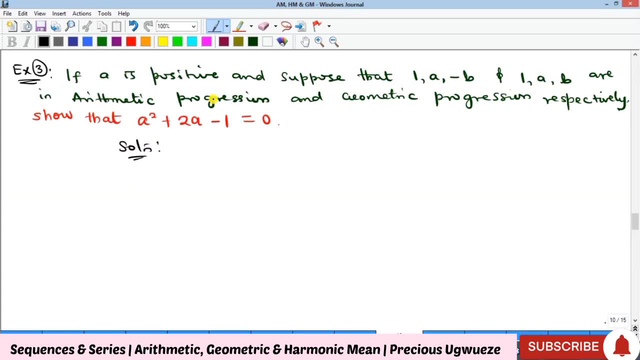 Okay, Our A, If A is A positive number, And suppose that This, This first sequence here, Is an arithmetic progression And the second Is a geometric progression, That we should show that This Will be true. Okay, 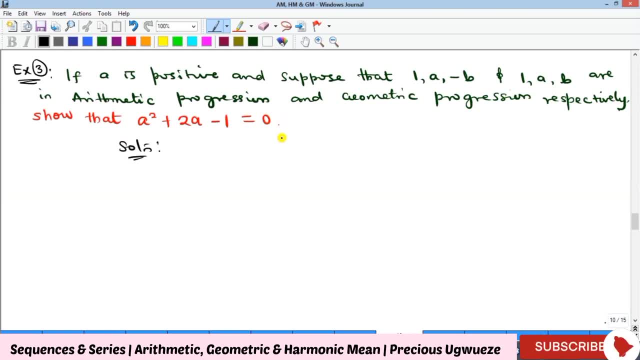 So Now We are going to apply both The knowledge of arithmetic mean And that of geometric mean, Assuming that here Is our A And this is C. So that means This is B. So by arithmetic progression, Our 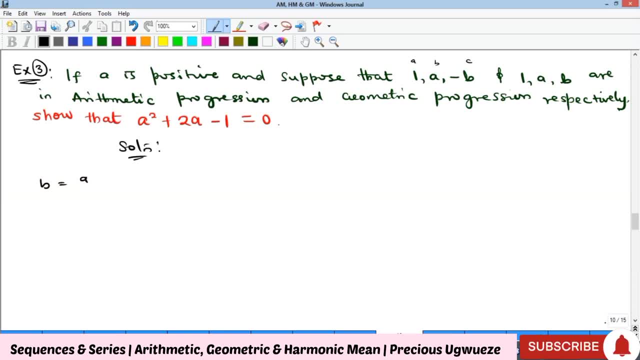 B Is equal to A Plus C All over 2.. So what it means Is that Our B In that Progression Is A. It must be equal to Our A, Which is 1..